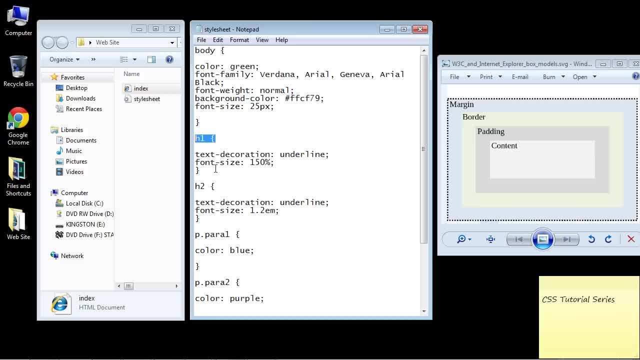 But they are there. They're just transparent. Think of it like that. But again, every single element will have four boxes around it and the content is the one we're using right now. So now, in order to see the content box, let's go ahead first and specify a background color. 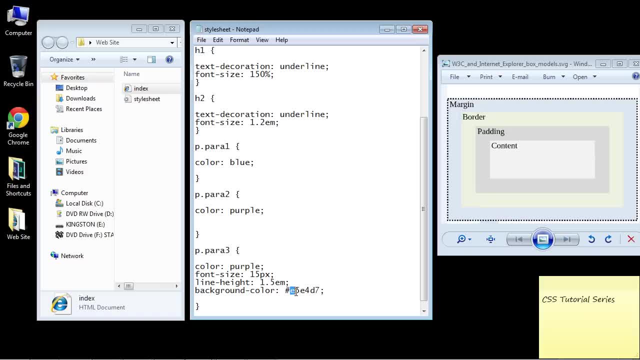 And we're going to go ahead and use a hexa code here. It's E5E4D7.. I actually like that color for my content boxes, So let's go ahead and save this And we'll open this up now, and there you can see everything that's. 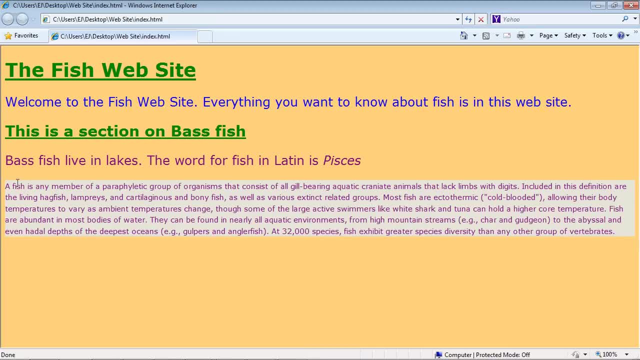 inside that color. That color that we just specified is our content box, And yeah, it looks like kind of a box, doesn't it? Now you'll notice how close the text is to the edge of the content box. So in order to increase that and give that a little space to make, 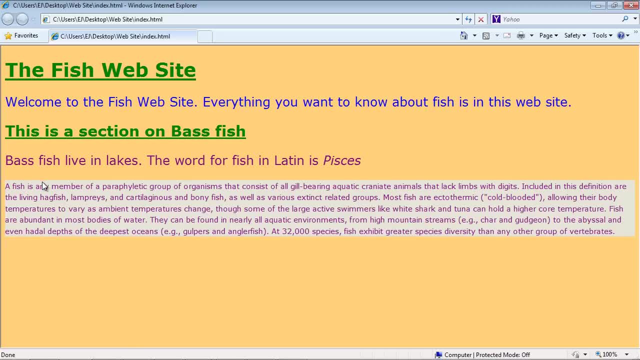 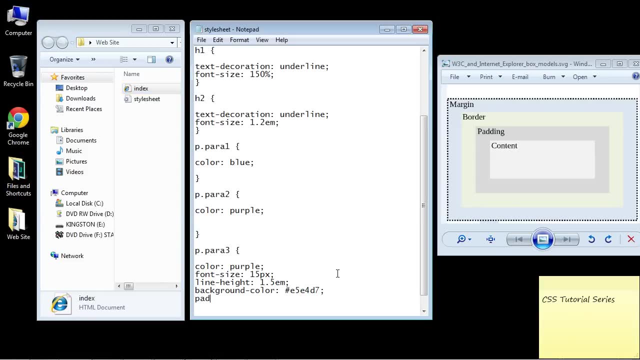 it look a little bit better. Let's go ahead and add some padding. So we're actually going to add the second box now. So let's close this out And we do that with the padding property. You guessed it- And let's give that 20 pixels. 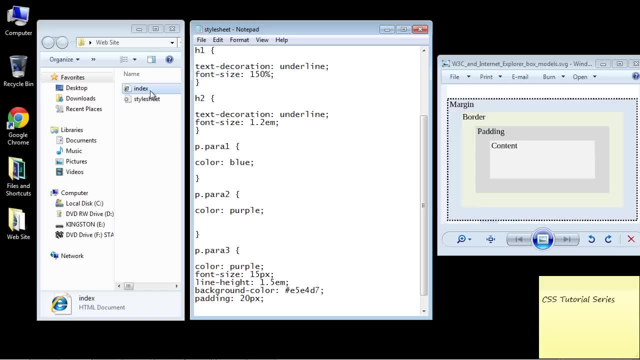 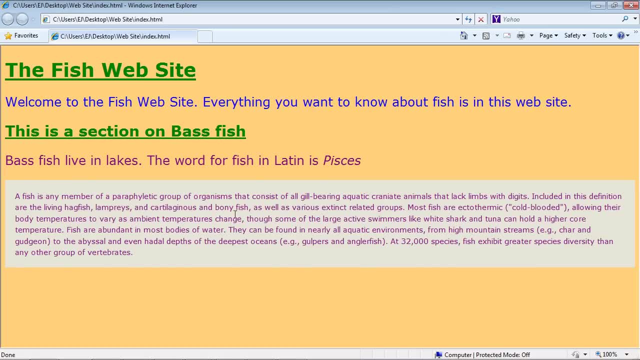 Let's go ahead and save this And let's open this up And there you can see we've got more space now. Look at that. And that looks a little bit better, in my opinion. Now let's add a border, So let's close this out again. 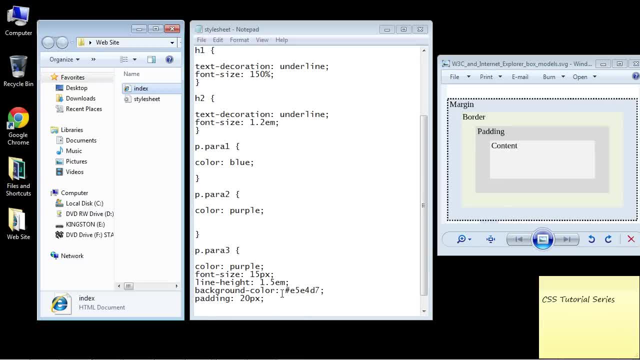 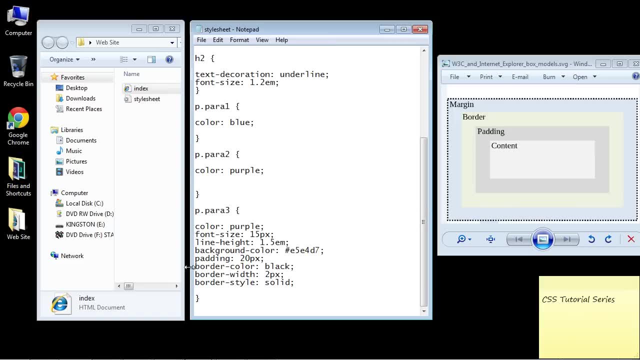 And that will of course, be the third box on this diagram. And to add a border. there are three properties for that, And I actually already typed these out, So I'm just going to copy and paste these in here. There is border hyphen color. 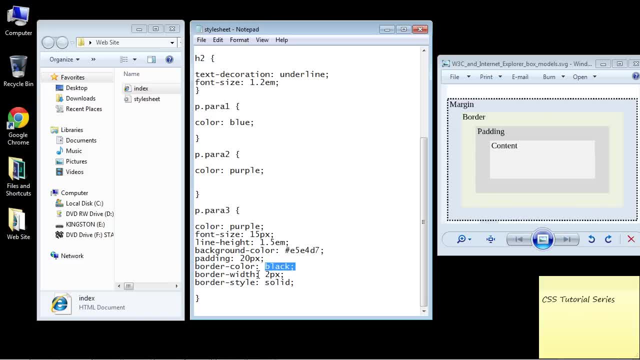 And we're going to make that black. That's pretty obvious. The border width, which we're going to make: 2px, And there's the border style which we're going to make solid, And in a future video I'll actually go over all the different parameters and values we can use for the border. 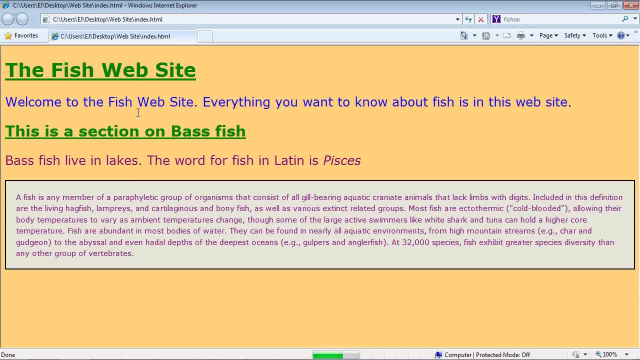 But for now, let's go ahead and save this And let's open this up And you can see we've got a black border. So we've got our content box right here, The padding, which is everything in between the content box and the border. 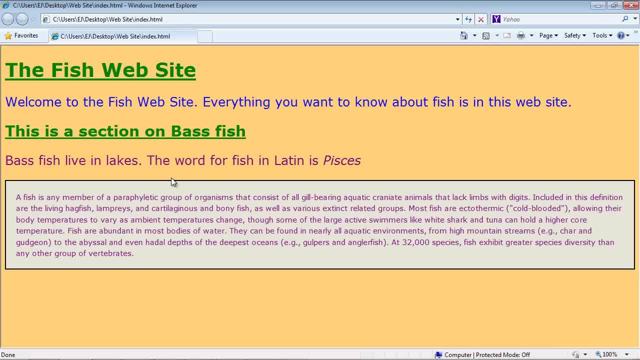 And then we have the border. So we have all three boxes. Now you might be asking what is the margin? The margin is this space right here. If you take a look on this left, that's the space between the side of the page and the border.